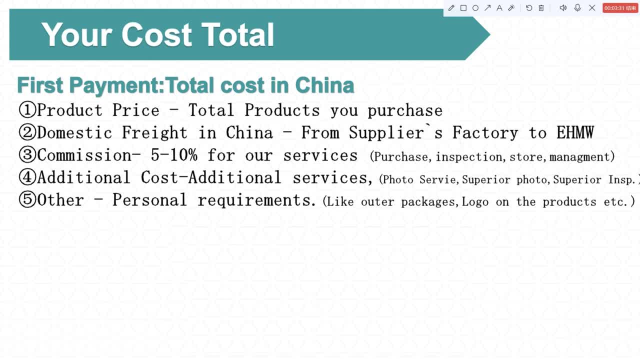 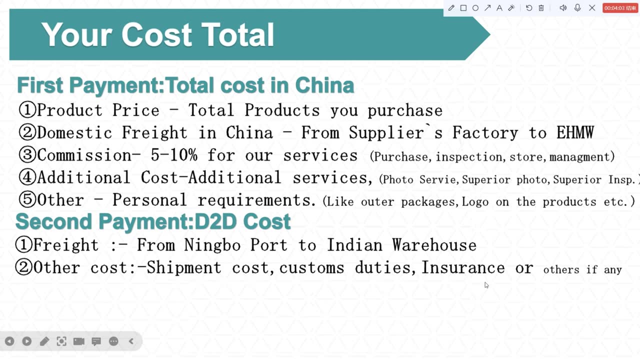 from our website. we charge some extra. Second payment is D2D cost. D2D cost includes the total freight from Nimbo port to Indian warehouse and other cost means the shipment cost, custom duties, insurance or any other. Third payment is domestic freight in India. Domestic freight includes: 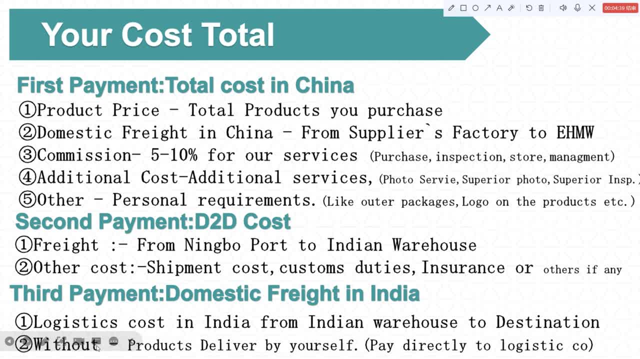 logistic cost in India from Indian warehouse to the destination. If you want, we can recommend you the third party logistic company to choose, or without, That means products delivered by yourself. These are the optional services. If you want, you can take this service from us or, if you want, you can hire a logistic team from outside and pay them. 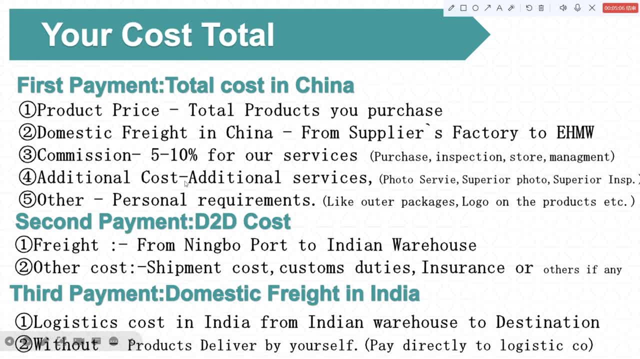 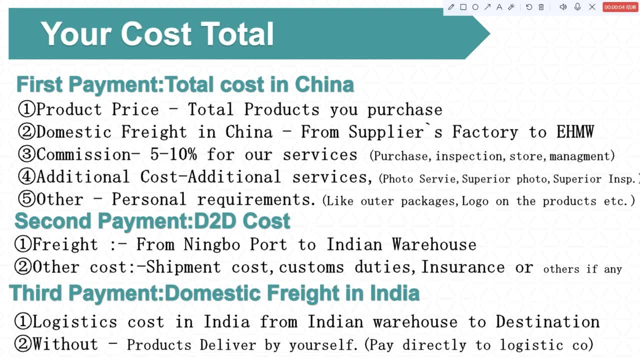 directly. If you choose our logistic team, we will ask the logistic company to check our delivery. in Sorry state, We will inform the customer service. who is scent? No Allah. respect the customer discounts. So these are the four benefits, along with the entire process. 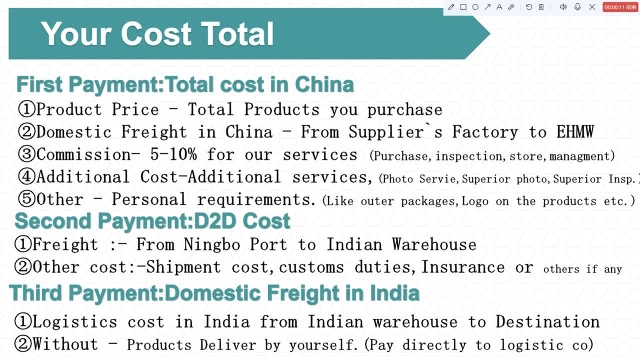 On the third export price. it includes all the DCT and conversion of product and shipping. Delivery can be from India to country or in India, or you can do truck phasing Iamente. this is India shipping. We are wonted to India so we have no확eder of India산. 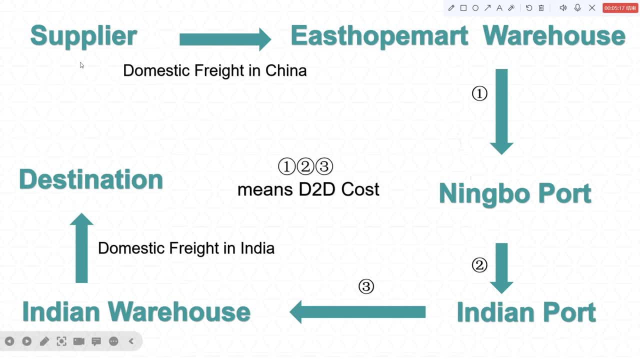 I want to show you one slideshow. So this is a slideshow from supplier to East Hope Türkiye warehouse, Which is our first payment. The second payment is from Nimbo port to Indian port. This is second payment. and from indian port to indian warehouse. this is our d2d cost from indian. 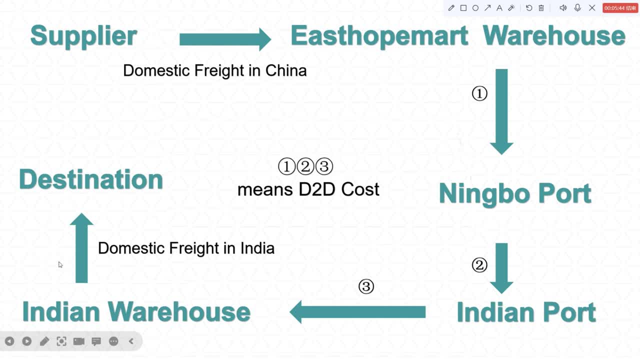 warehouse to destination is optional. we have this facility in india also. if you choose, our service is okay. if you want, you can choose your own company from outside. this is our slideshow to show you our d2d cost when you place an order and confirm that you want to buy the products. 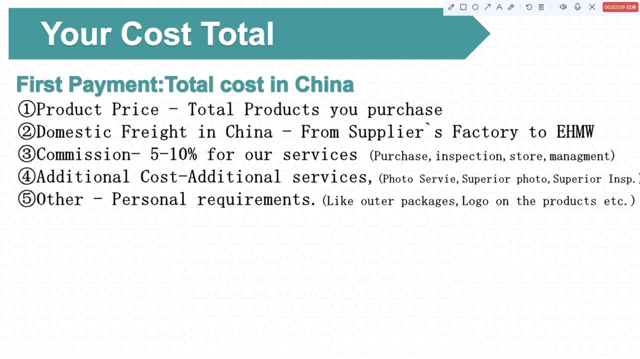 you have to contact our indian partner for the payments. once you complete the first payment- that is total cost in china- only then we can buy your products from the supplier and load them to india. after goods arrive at indian port, our indian partner will notify you to pay d2d cost. 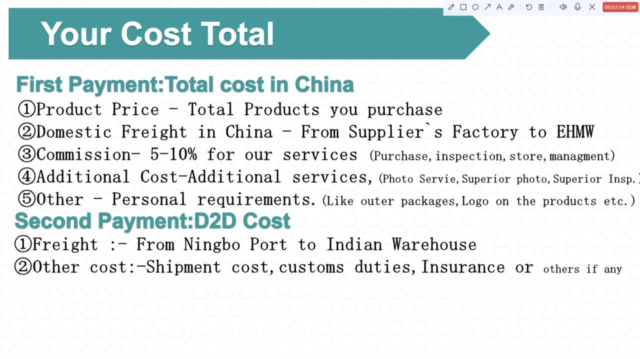 and the domestic freight. you have to pay the d2d cost within seven days. you are not able to make a data change to the d2d fahren. we have the complete 다고겠다고 했고요. this is our final payment. by the way, price on schafer to permit.